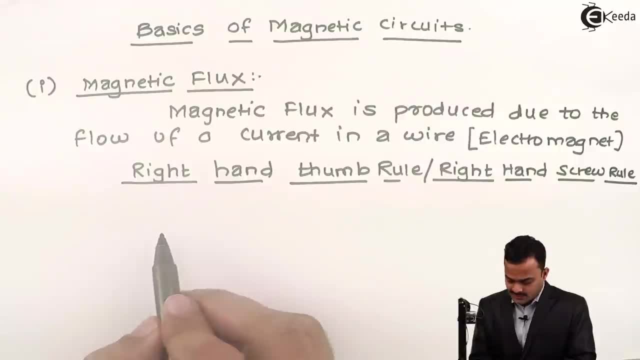 So, roughly if I draw the sketch, if I consider this is a conductor holding in right hand such a way that 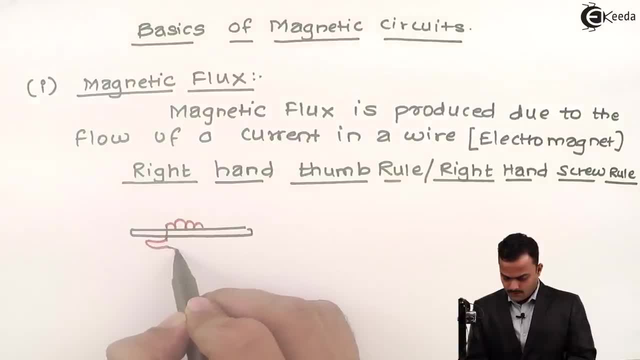 outstretched thumb will give you the direction of electric current passing through it. 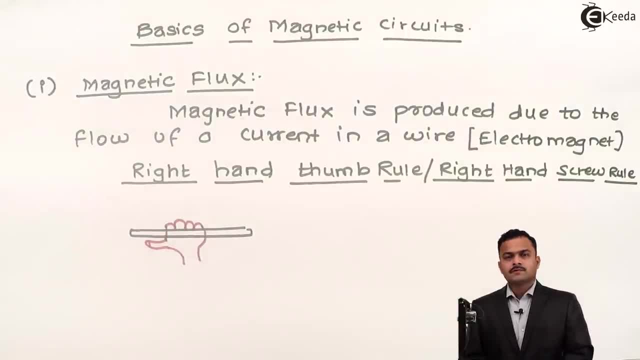 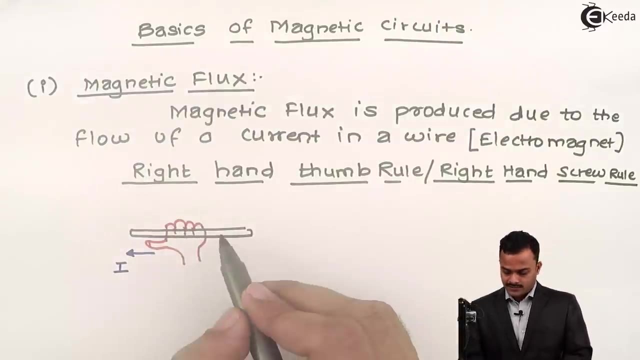 So, I will consider this as a right hand and this is a thumb outstretched. Then, if that outstretched thumb is determining the direction of current, then curl fingers around a conductor will give you the direction of magnetic flux. So, the direction of magnetic flux will be like this. 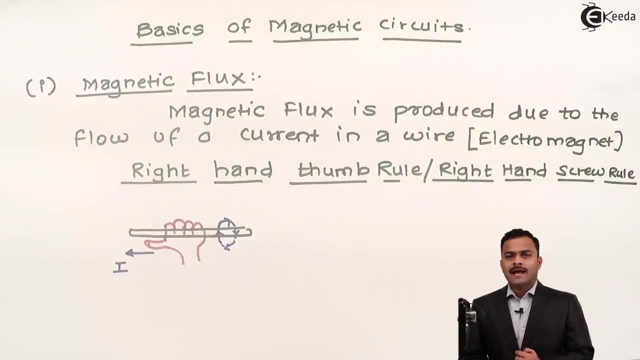 And this will be the line of electromagnetic flux. So, these lines are a closed circle. Hence, it will be like this. In other words, I can get the direction of magnetic flux by right hand screwing. So, this is the screw rule. What it says? Suppose, you are fitting a screw and considering that you are using a right hand. If I give the rotation in clockwise direction, then screw will go inside of the wall or a wood or a paper for that matter. 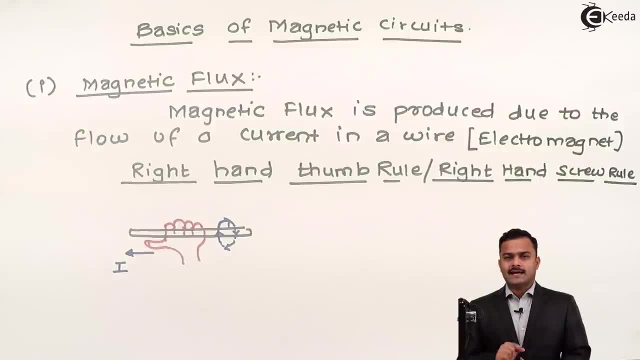 Then, if that going inside will determine the direction of current, then the rotation of a screw will give you magnetic flux. I repeat. 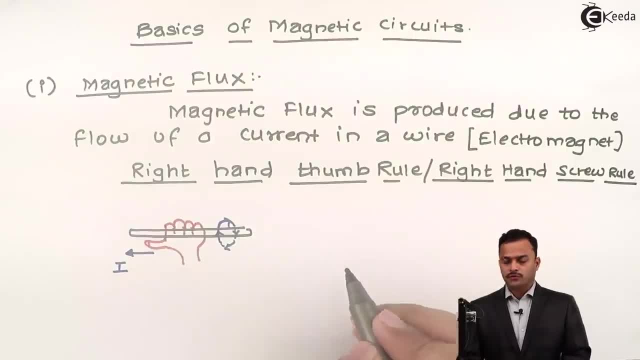 Suppose, I am having a screw which I want to fit inside this paper. And that is determined by this cross. So, cross is nothing but going inside. So, if this determines the direction of current, then in order to get screw inside the paper, I need to have a clockwise motion or clockwise torque. 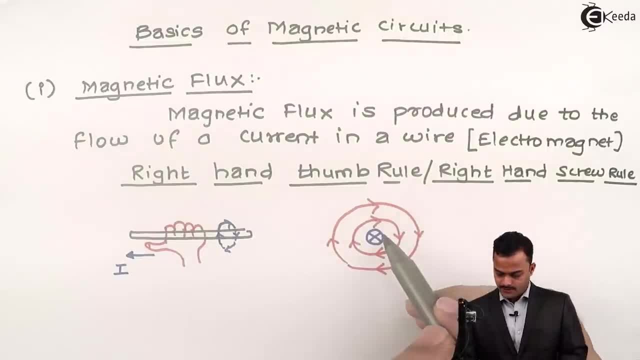 So, this is a direction of current. So, this is a direction of current. So, this is a direction of current. 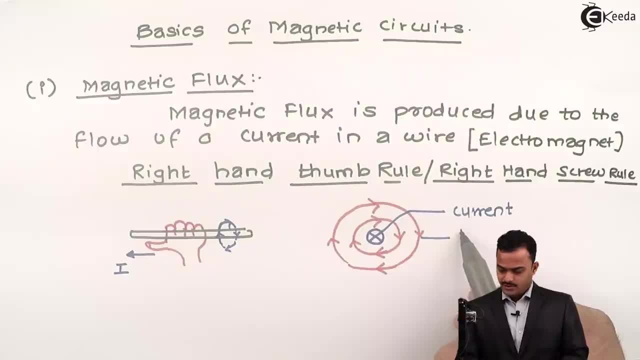 And this is nothing but direction of magnetic flux. 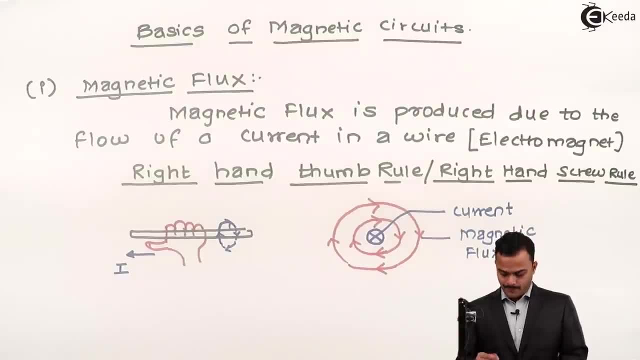 Similarly, if you want to take a screw out of the paper, that is represented by dot. 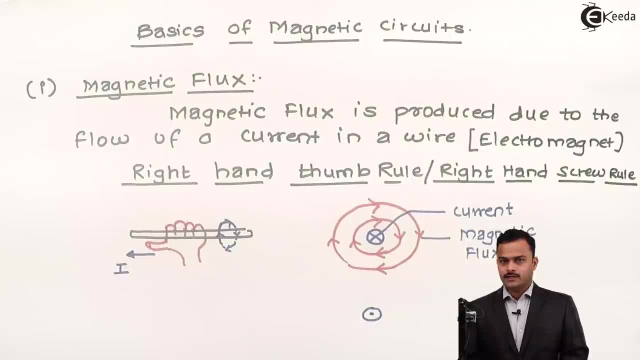 So, obviously I should have an anti-clockwise torque given to this screw. So, it will be like this. 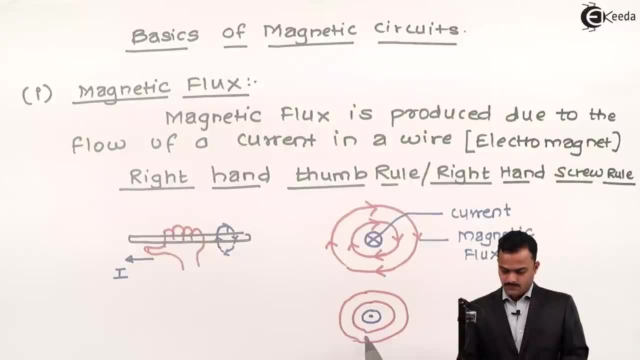 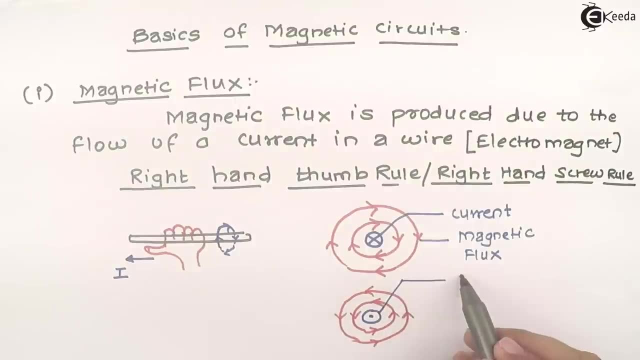 So, once again, this is the direction of current and this is the direction of magnetic flux. 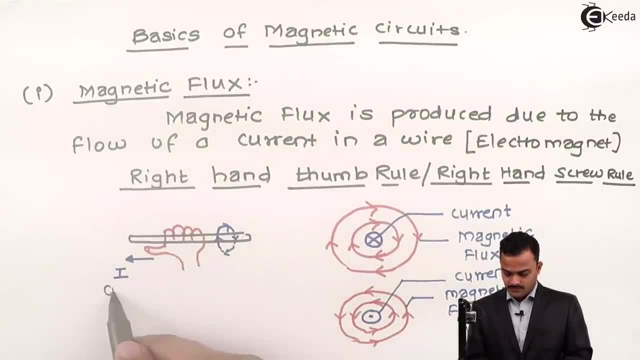 So, over here, to right hand thumb rule, this is a current and this is a magnetic flux. So, over here, to right hand thumb rule, this is a current and this is a magnetic flux. 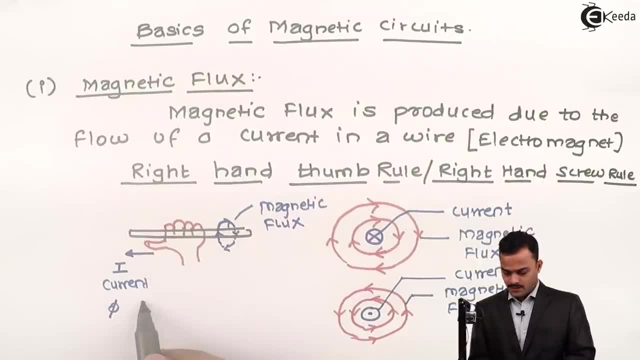 Magnetic flux is denoted by letter phi and unit is Weber written as WB. 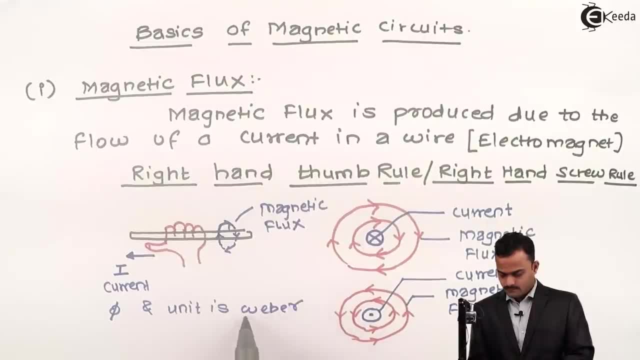 Magnetic flux is denoted by letter phi and unit is Weber written as WB. 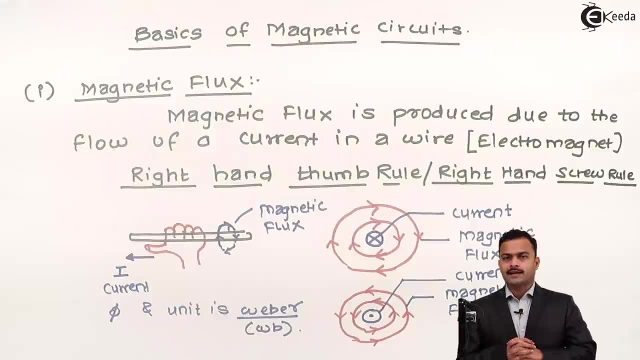 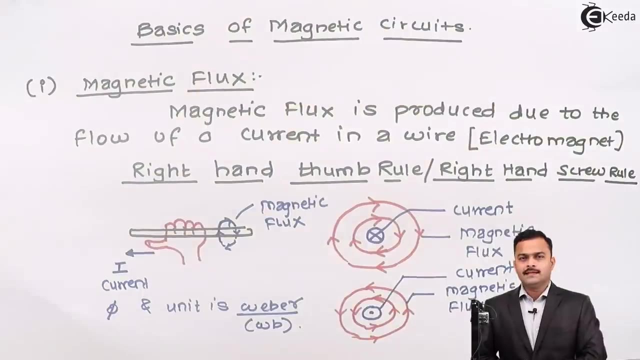 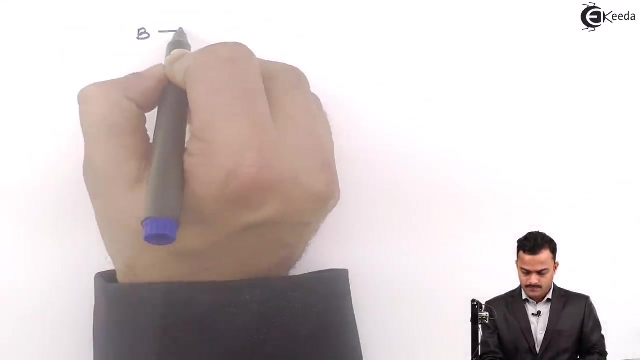 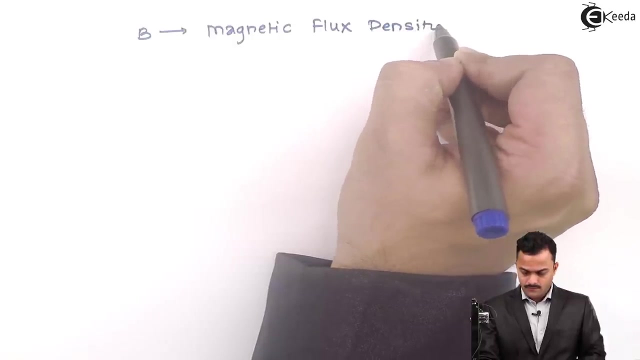 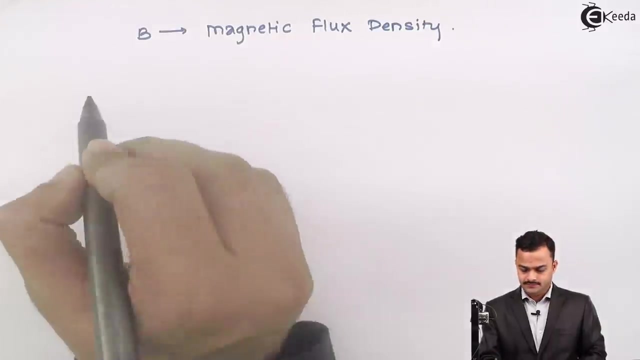 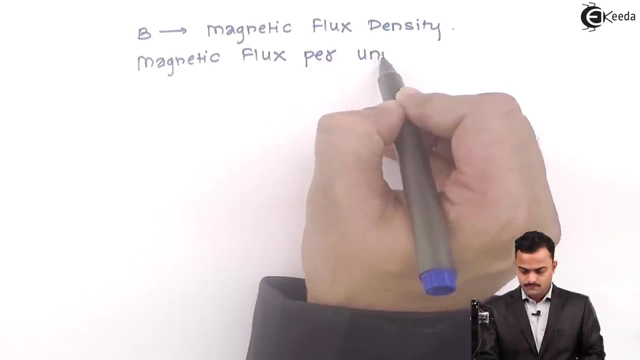 So, whenever there is a current flowing through a conductor, magnetic flux is always associated with that. And the direction of this magnetic flux is determined by right hand thumb rule or right hand screw rule. Normally, magnetic flux is represented by flux density and it is denoted by B. So, B is the flux density. And it is defined as magnetic flux per unit area. 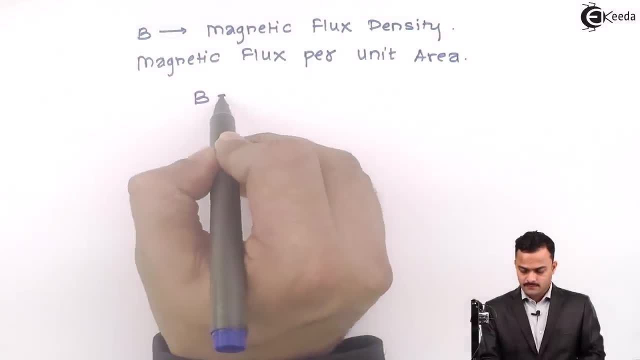 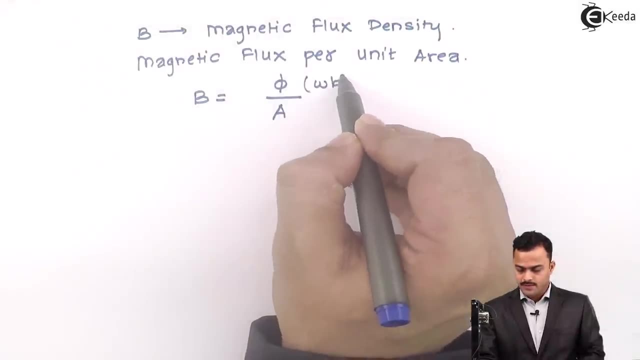 So, B is given. B is given as phi divided by A. The unit of phi is Weber and unit of area is meter square. 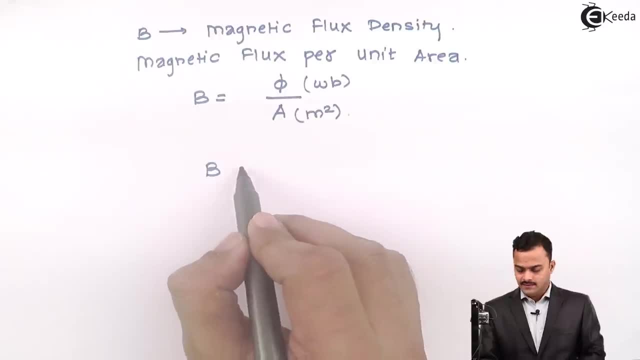 Hence, magnetic flux density will have the unit Weber per meter square. So, for each and every magnetic material, its property can be determined. By B which is nothing but magnetic flux density. 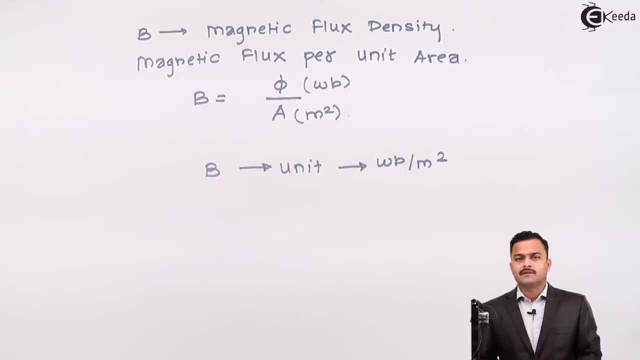 Let's go to the second concept and that is MMF. Which stands for magneto-motive force. 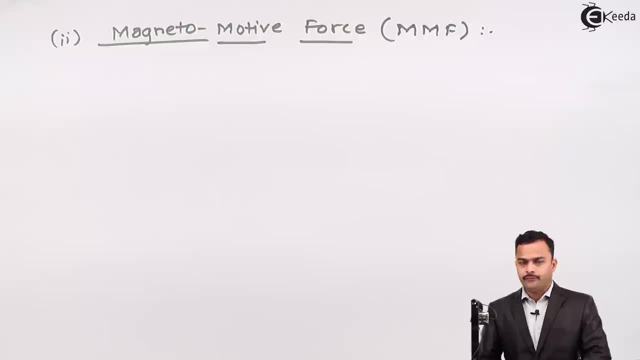 It is analogous to electro-motive force. Which is nothing but EMF in electric circuit. 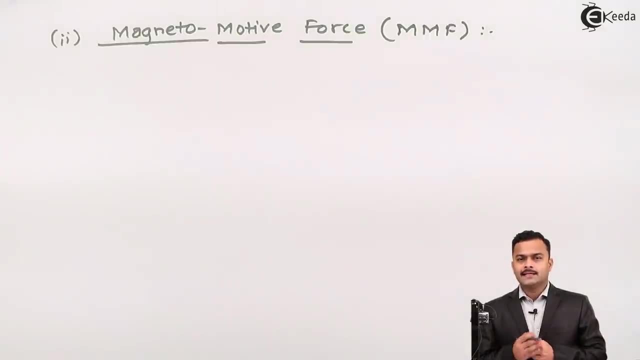 So, MMF is nothing but ability to produce magnetic flux. So, we have seen that magnetic flux is produced due to electric current passing through a winding. Hence, number of turns of the windings comes into the picture. And then current passing through it. Both together are responsible to produce a flux. Hence, I can say magneto-motive force MMF is nothing but N into I. 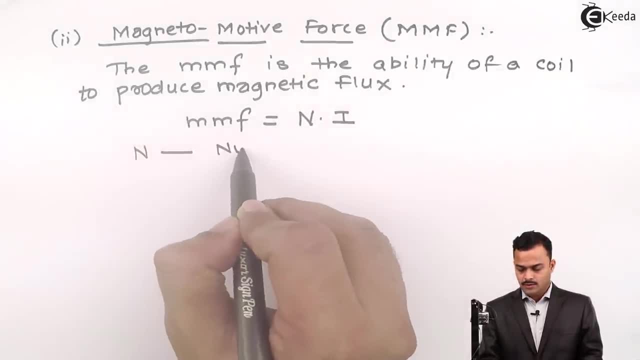 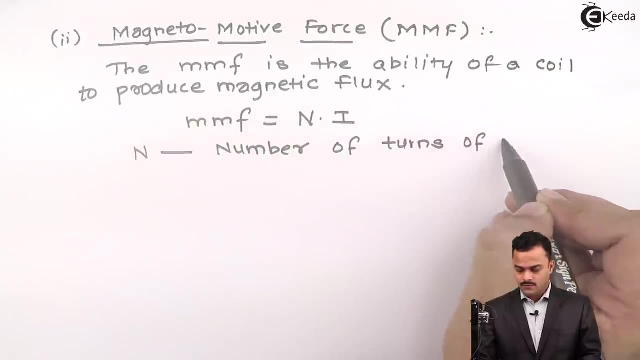 Where N is the number of turns of winding in a coil. And I is nothing but electric current passing through. Current passing through coil. 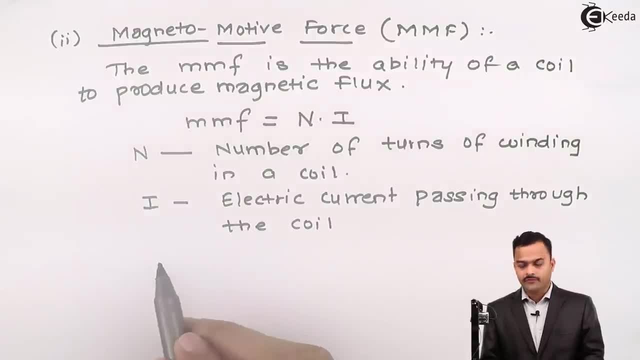 MMF is denoted by F. 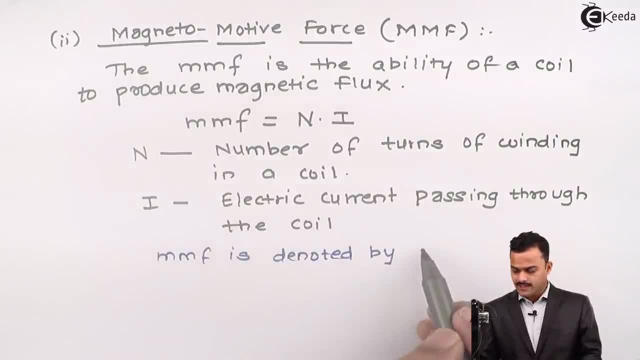 It is not like our force. Therefore, MMF is having symbol like this. We call this as F. But the symbol will be like this. And unit of MMF is derived from this formula. 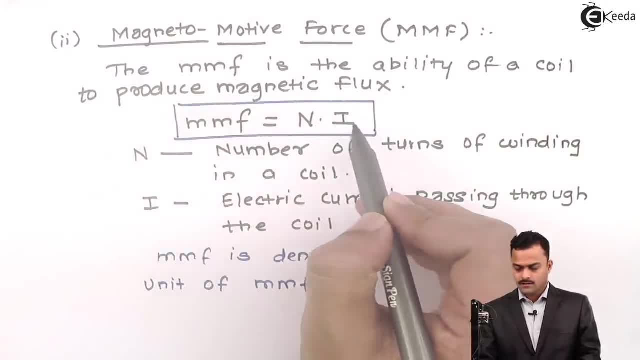 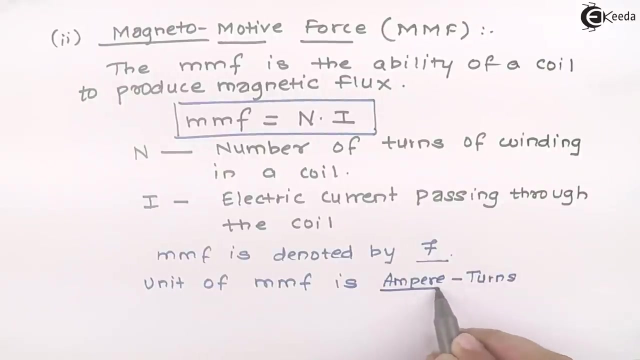 I into N. I's unit is ampere. And N, number of turns. Hence, I can call this as turns. So, basically the ampere turns. In short, I can say it is ampere turn or AT. So, AT stands for ampere turns. Let's move to the next concept which is magnetic flux intensity. 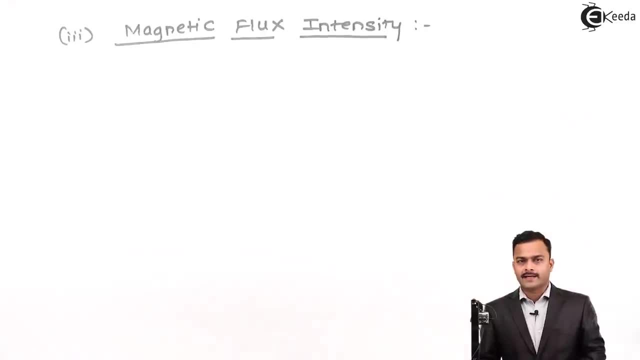 Another important property of a magnetic material. 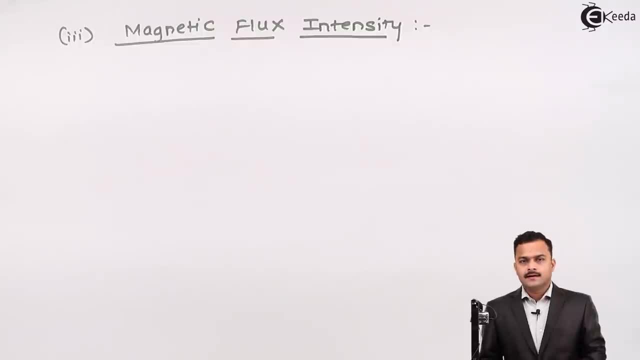 Which defined as magneto-motive force per unit length. 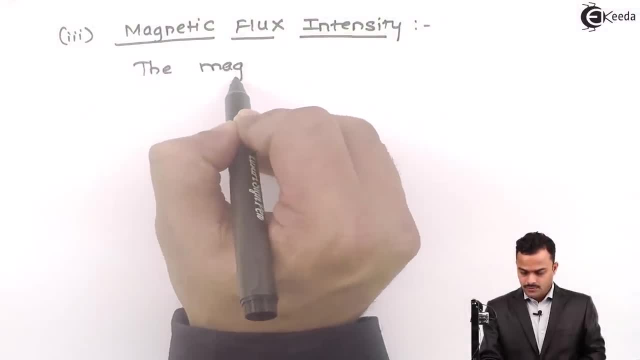 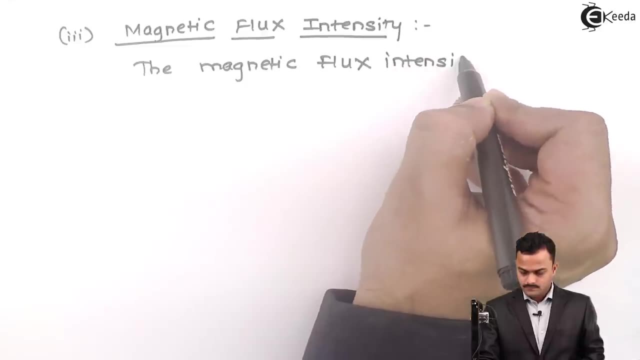 So, the magnetic flux intensity is the MMF or magneto-motive force. Per unit length. 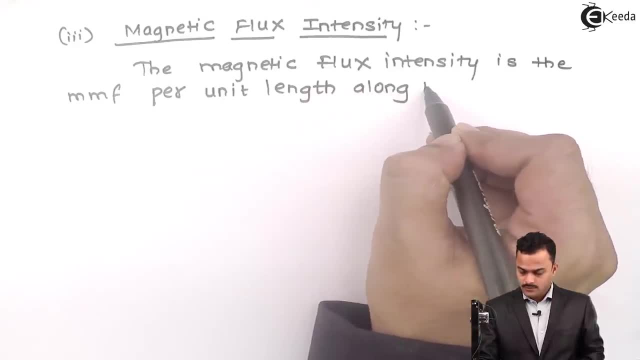 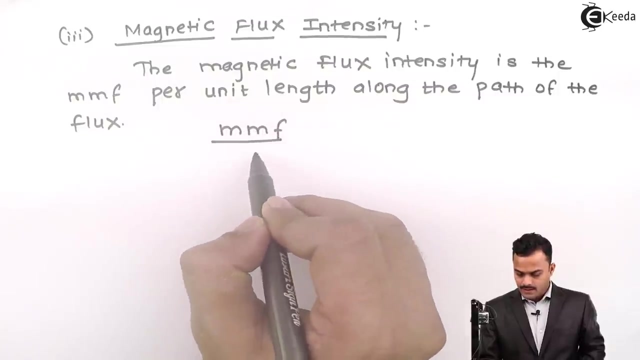 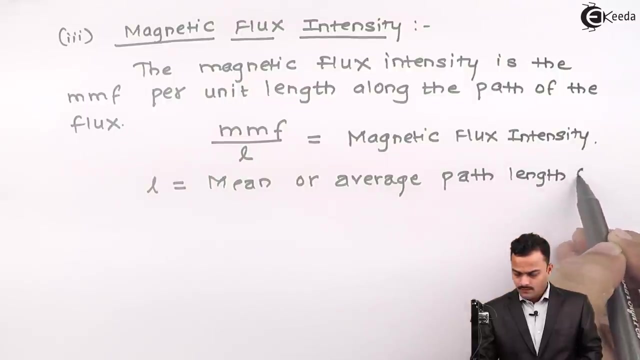 The length is along the path of flux. Hence, it is given as MMF divided by length L. Which is nothing but. Magnetic flux intensity. Where L stands for mean or average path length of the magnetic flux. So, it is a length. 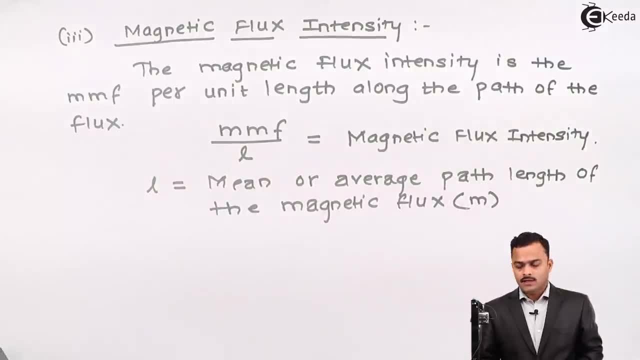 Hence, unit is meter. And magnetic flux intensity. I will write over here. It is magnetic flux intensity. Is denoted by symbol H. Hence, I can say H equal to. MMF. MMF. Upon L. 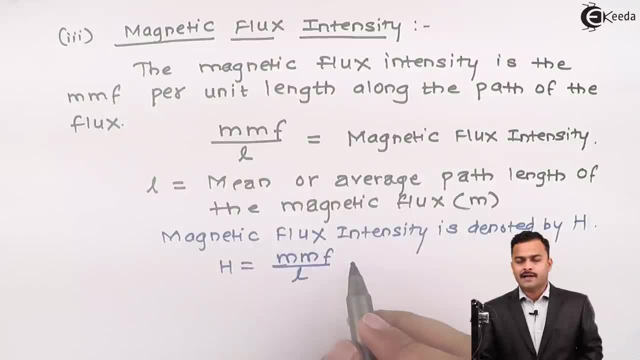 MMF is nothing but. Number of turns multiplied by electric current I. 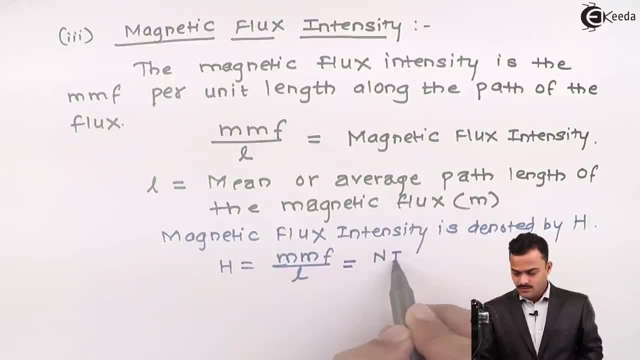 NI. So, the formula of H is NI divided by L. 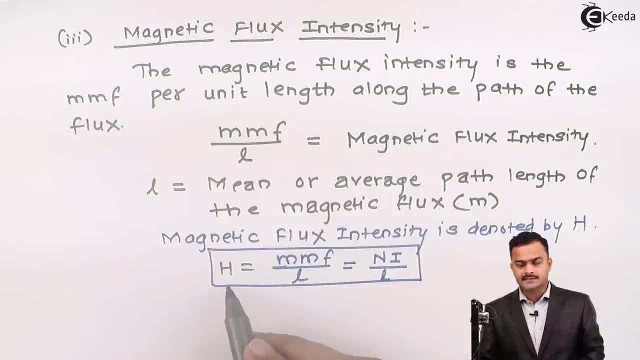 From the formula, we can derive the unit of H. So, NI is ampere turn. And length will have the unit meter. 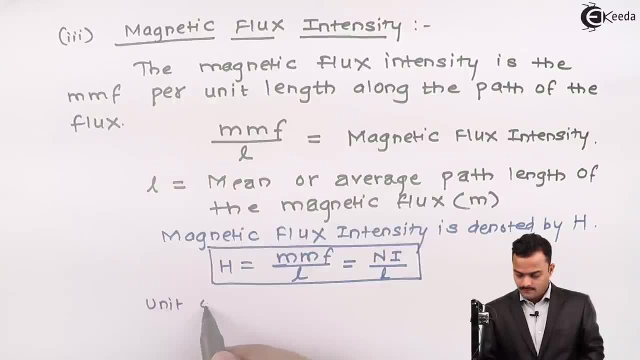 Hence, I can say unit of H is ampere turn upon meter. So, you can say ampere turn per meter. 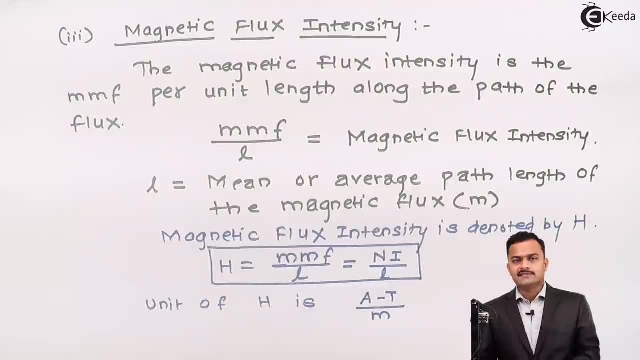 So, this is all about magnetic flux intensity. Let's move to the next concept and that is reluctance. 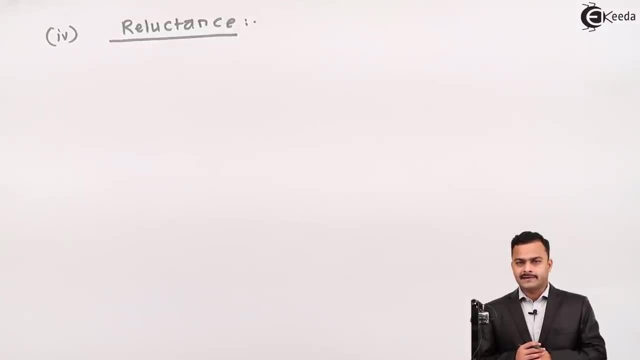 It is analogous to resistance in electric circuit. And we state it is the opposition offered by a coil to magnetic flux. 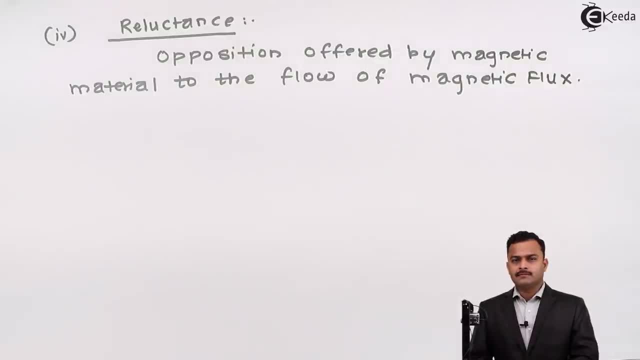 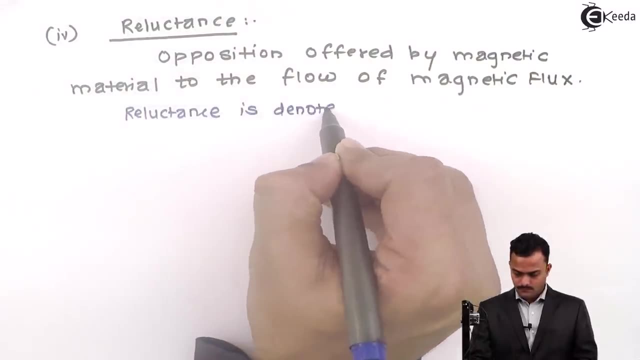 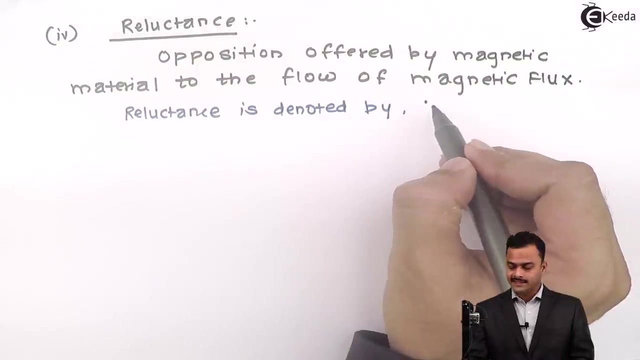 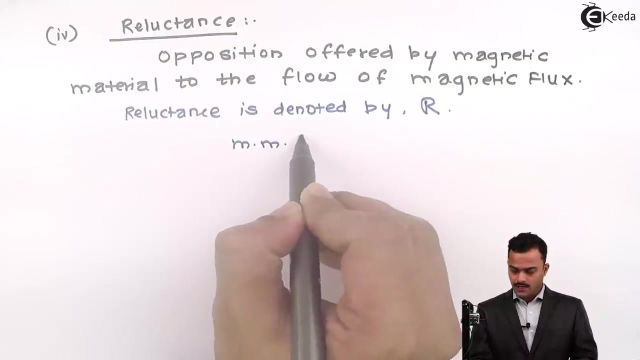 The reluctance can be denoted by R. But, this R is different than that of an electric circuit resistance. Hence, it is denoted as R and written like this. The relationship between MMF flux and reluctance is governed by this equation. So, MMF equal to reluctance multiplied by flux phi, where reluctance is given by the formula 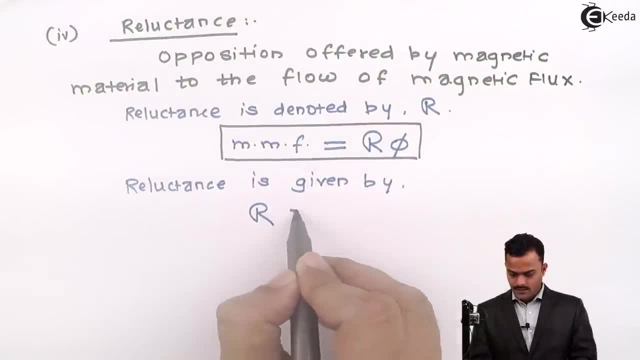 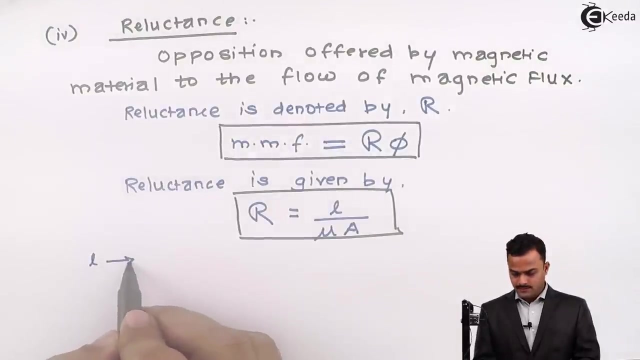 R equals L divided by mu into A, where L is nothing but the average length of the magnetic core. So, this is the length of the magnetic core. So, this is the length of the magnetic core. 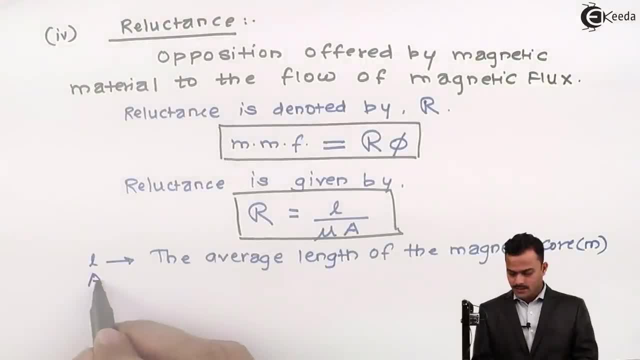 Since it is a length, hence unit is meter. And, A is area of cross section of the core. 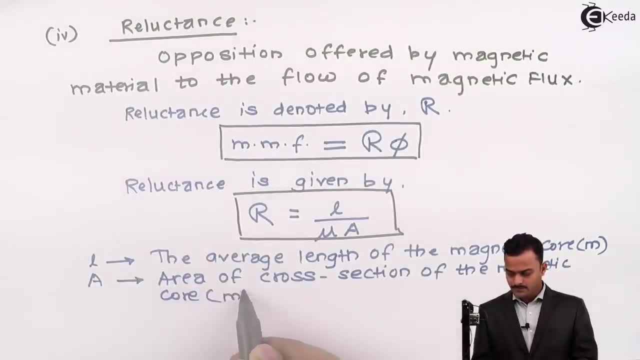 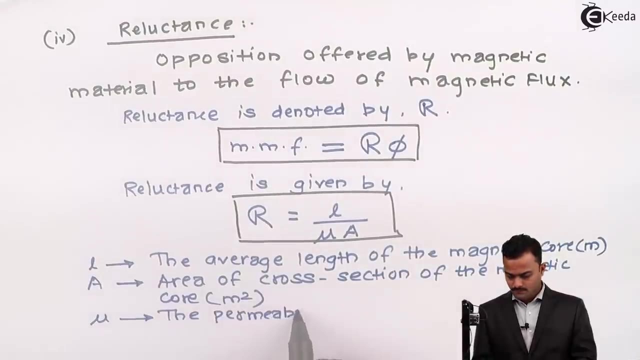 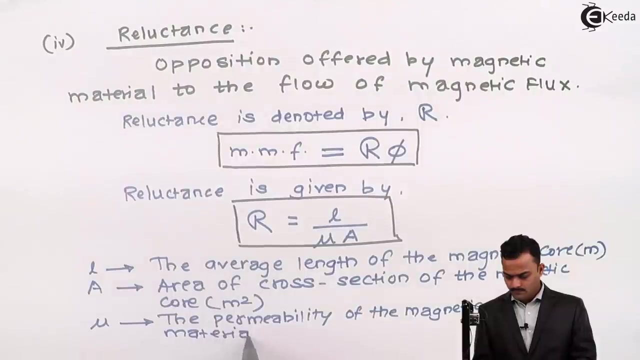 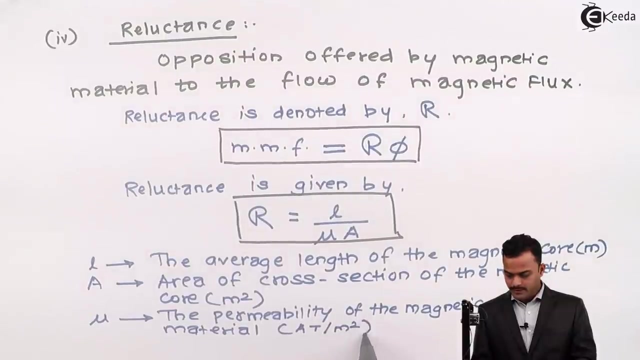 So, being an area, the unit will be meter square. And, now one more property of a magnetic material, nothing but mu, which is nothing but permeability of the material. So, being an area, the unit will be meter square. And, now one more property of a magnetic material, nothing but mu, which is nothing but permeability of the material. called as a permeability. It is just similar to that of a conductivity in case of electric circuit. 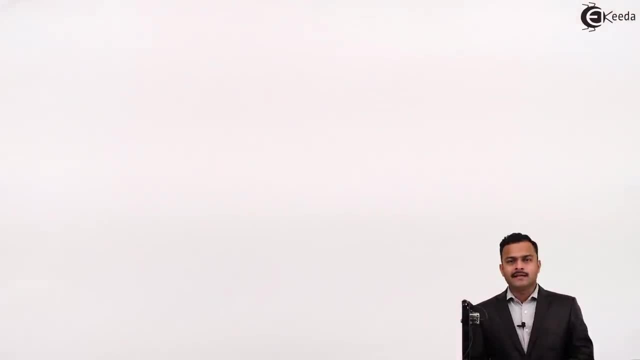 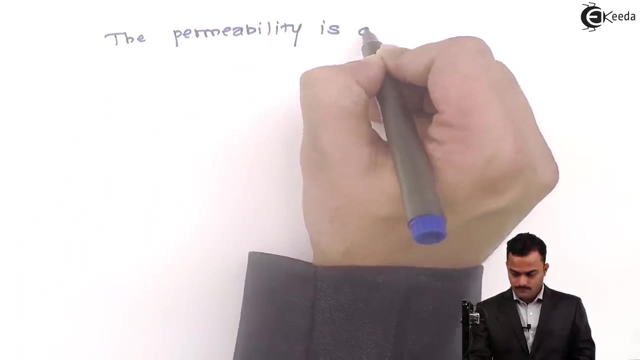 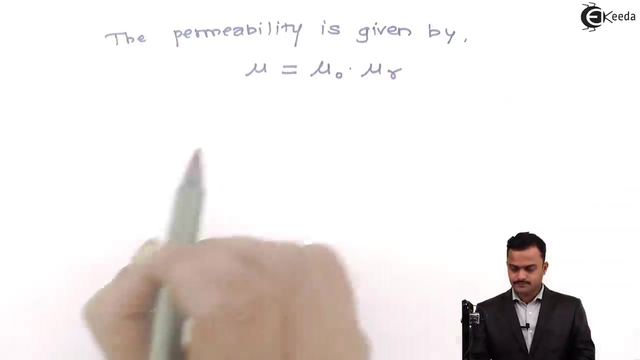 Okay, permeability is given by mu equal to mu naught into mu r where mu naught is the permeability of the air. 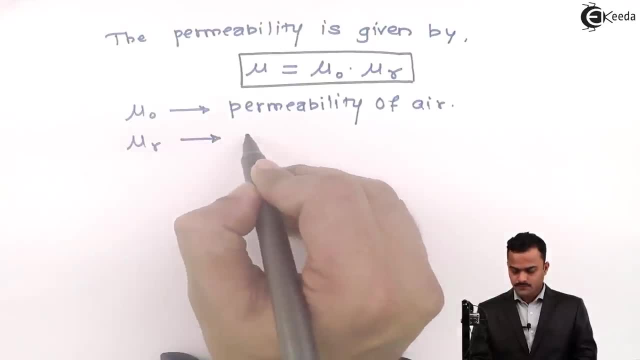 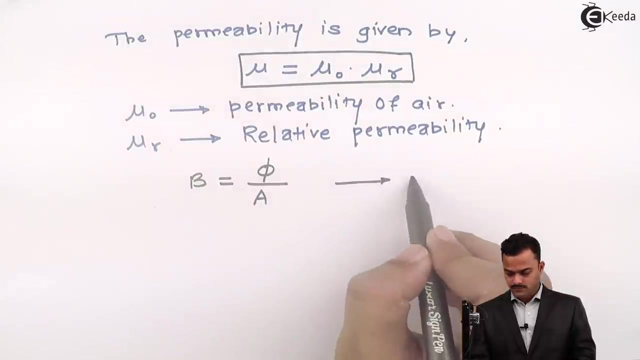 And mu r is relative permeability. Now, let us consider the magnetic flux density which is given by b equal to phi upon a. First equation. Now, basically what we are doing, we are going to establish one relationship. Between b, mu and h. Doing so, we are going to revise all the formulas of repeat formula also. 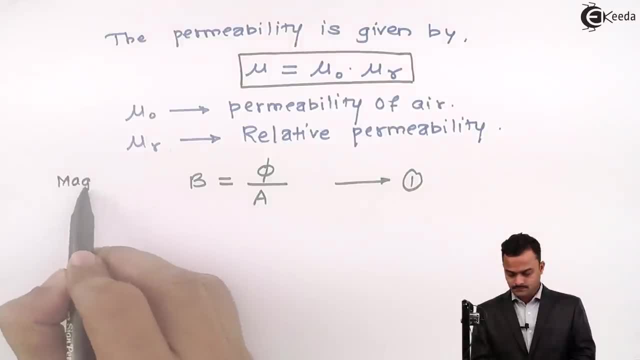 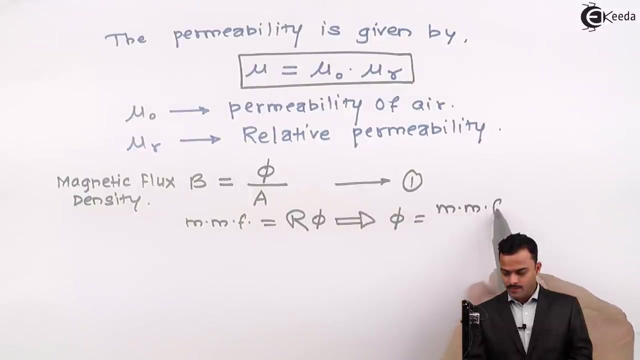 So, b is what? Magnetic flux density. Now, we know MMF is nothing but reluctance r multiplied by flux phi. This implies phi equal to MMF upon reluctance r. 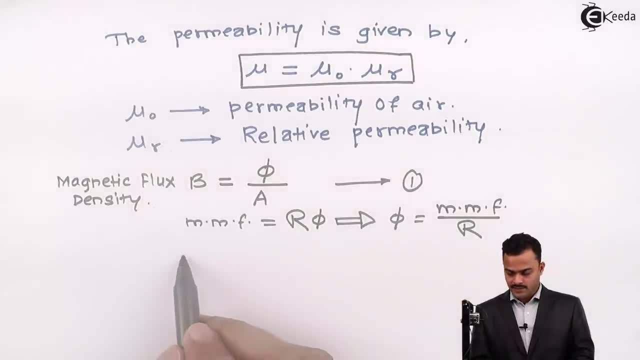 So, I am going to substitute this over here. What I will get? b equal to MMF upon reluctance r divided by area a. MMF. So, I will consider this as equation number two. MMF is a into i. So, once again write over here. MMF is magnetomotive force which is responsible for production of magnetic flux. 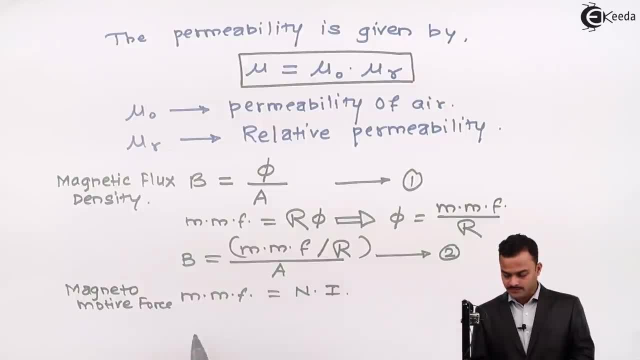 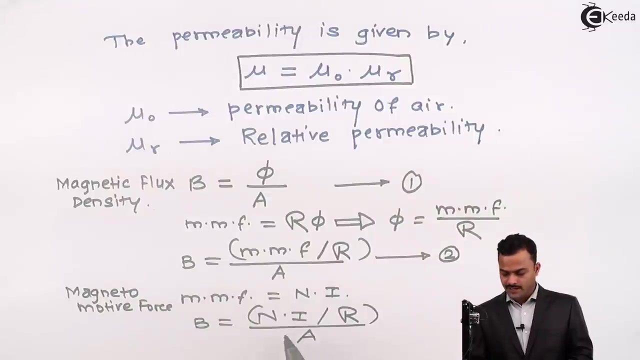 One more substitution I am going to make over here. So, b equal to ni divided by reluctance r divided by area a. So, I will get this relationship. Now, we know. Now, we know reluctance is given by r equals. 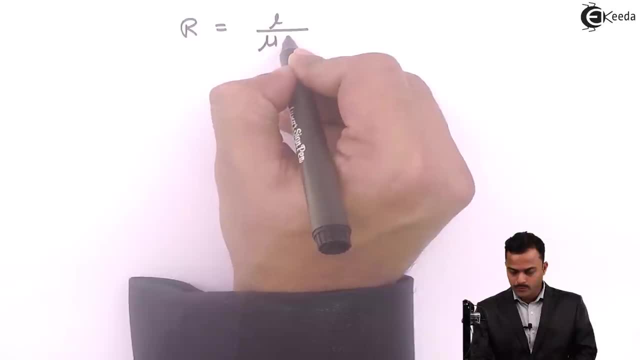 L upon mu a. So, this is the formula of reluctance. 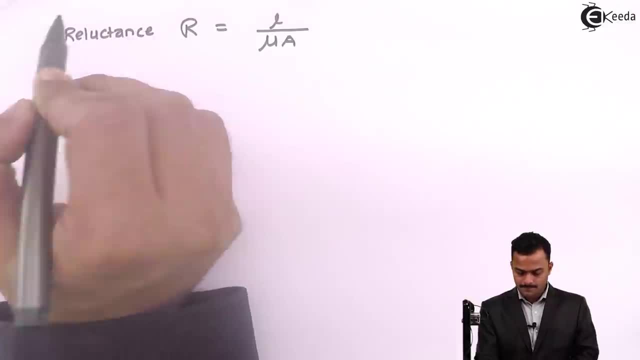 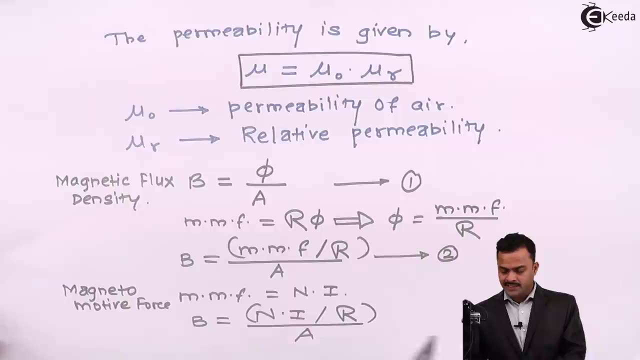 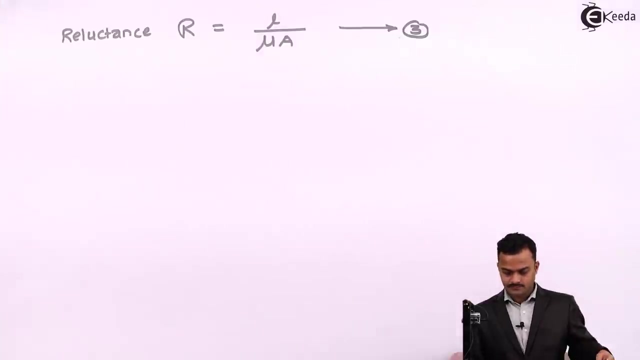 Now, I will substitute this equation in the equation that we derive for magnetic flux density. So, what I will get? b equal to. 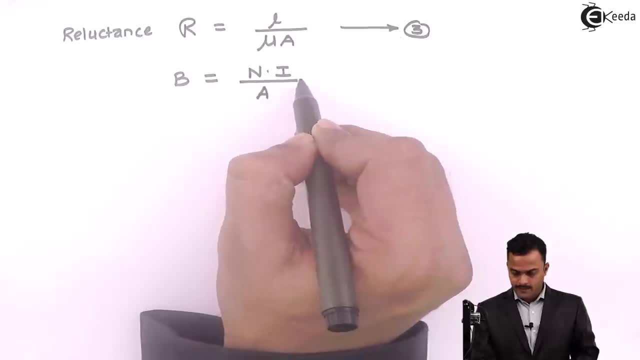 Ni divided by a. And reluctance is in the denominator. 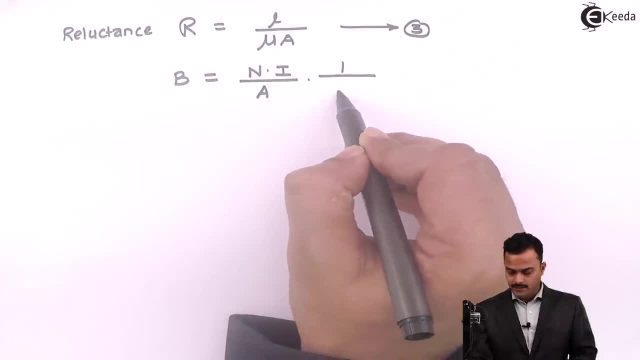 Hence, 1 divided by L upon mu a. 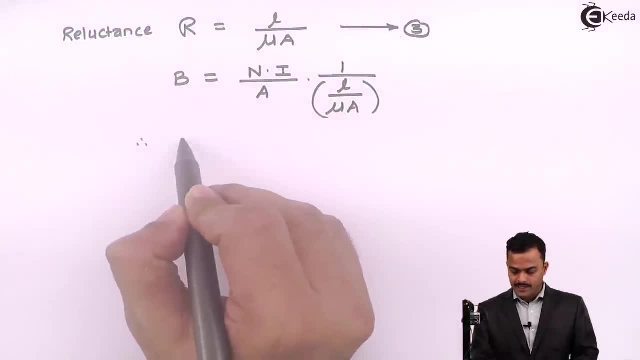 If I rearrange the terms, what I will get? b as n into i upon a. multiplied by mu a. 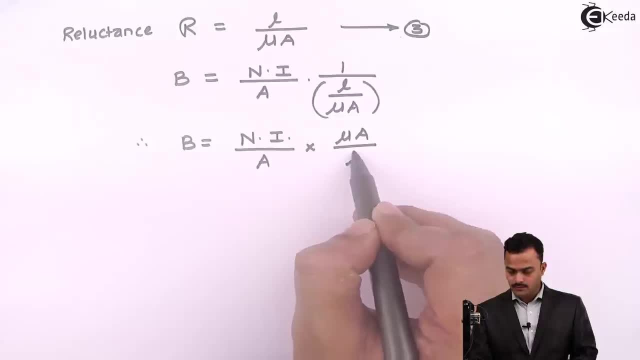 mu a upon l. I can cancel this a. Finally, I will get b as ni upon l multiplied by mu. 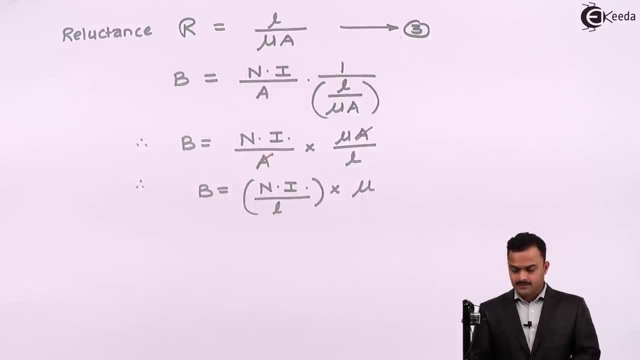 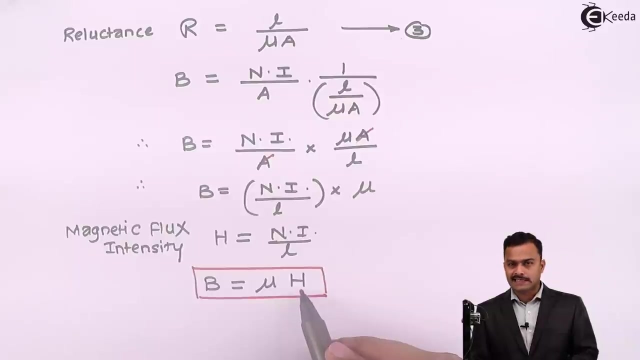 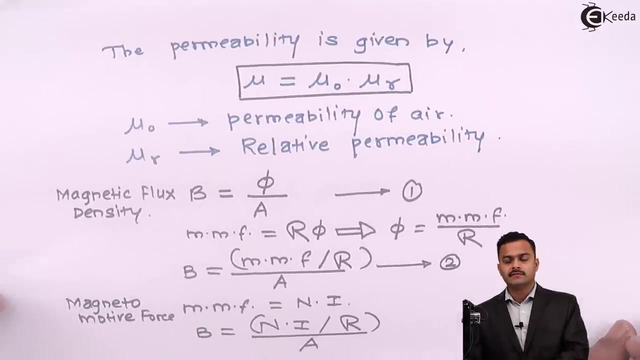 Now, we have seen that mmf per unit length is nothing but magnetic flux intensity. So, I can write over here magnetic flux intensity which is denoted by h is nothing but ni upon l. And if I substitute this over here, I will get b equal to mu into h, a very important relationship between magnetic flux density and magnetic flux intensity. Now, in this derivation, important formula we have seen. So, the first formula is for a magnetic flux density. 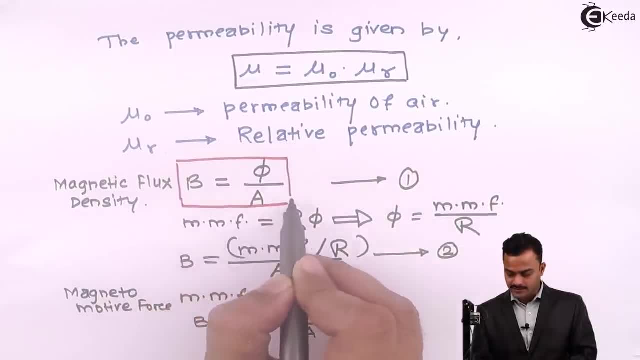 . It's a kind of a revision of a magnetic circuit. Flux per unit area. Then, we have seen second 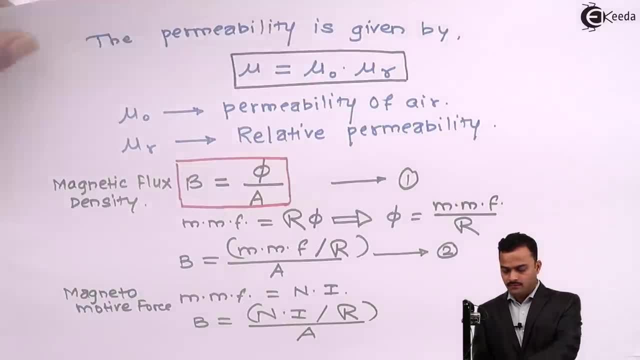 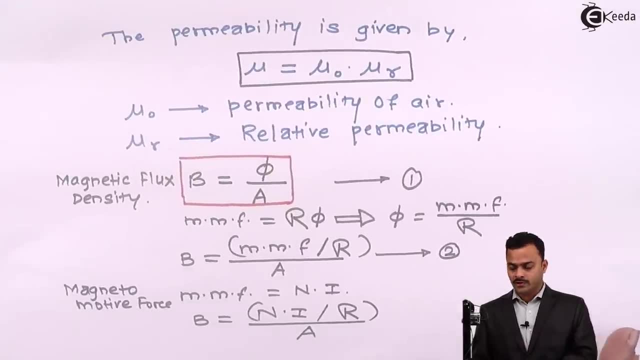 important formula of mmf. And actually, mmf is a magnetomotive force nothing but n into i. . 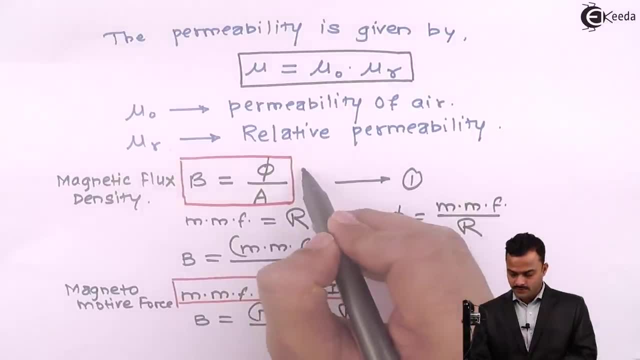 So, let the units also. . This unit is Weber per meter square for magnetic flux density. For magnetomotive force, it